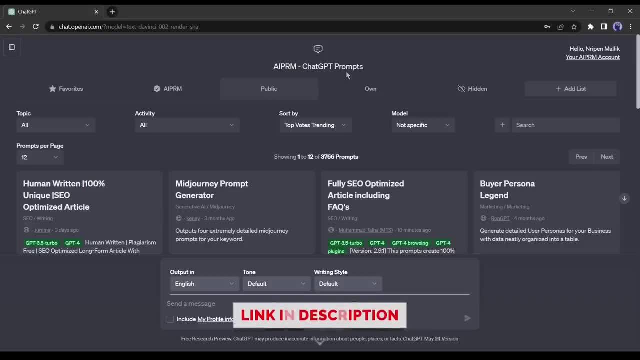 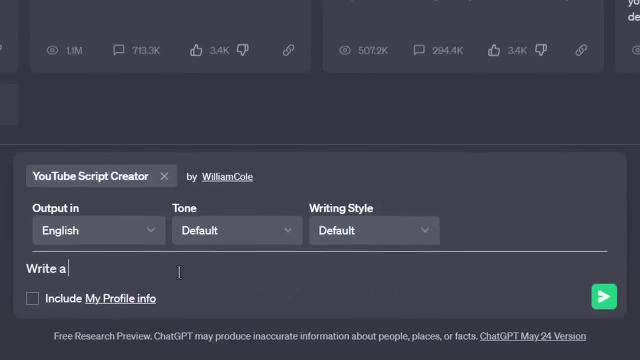 If you're unfamiliar with Aperm, you can watch one of my previous videos where I explain how to use it. Once you have installed Aperm, you can use the Aperm Prompt Guide. You can also use the Aperm App, find the YouTube script generator and provide the prompt. write a child learning video. 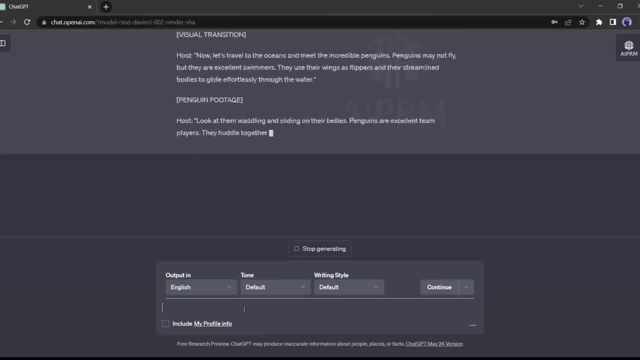 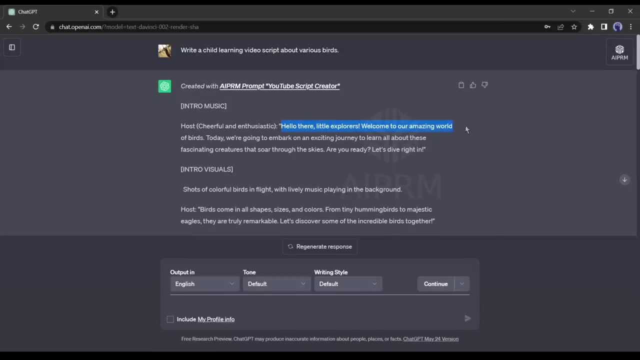 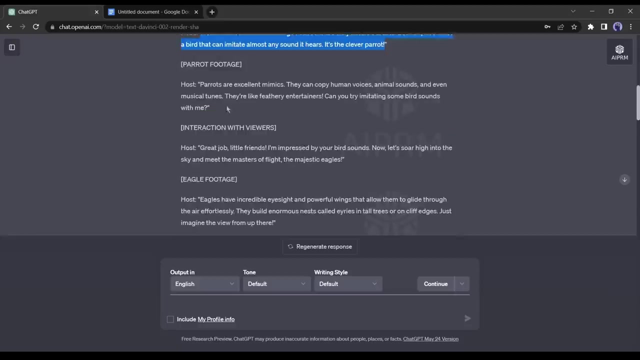 script about various birds. ChatGPT will generate a captivating YouTube video script with proper instructions about visuals and content. Copy only the host part of the text and paste it into a document file such as Google Docs. Then copy the entire script and paste it into the same document. 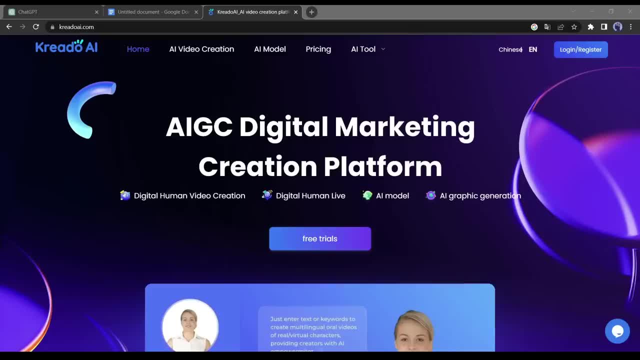 file. This completes our first step. In the second step, we will generate the voice for our video using a text-to-speech AI. We will also create a voice for our video using a text-to-speech AI. In the second step, we will generate the voice for our video using a text-to-speech AI. We will also 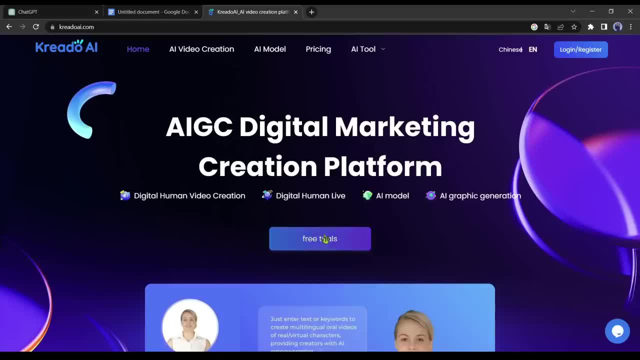 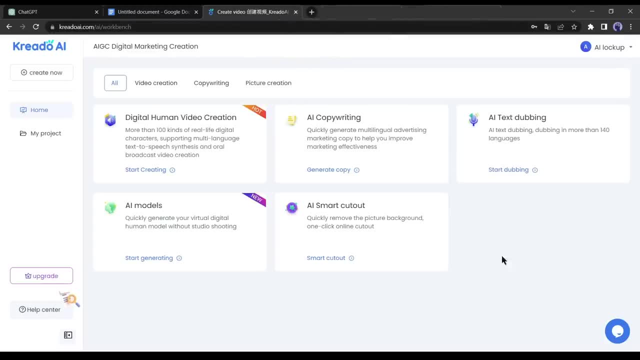 create a voice for our video using a text-to-speech AI called Credo AI. If you are new to Credo AI, click on Free Trial and create an account with your email and password. Verify your email address after successfully creating the account. Once you're logged in, click on AI Text Dubbing and. 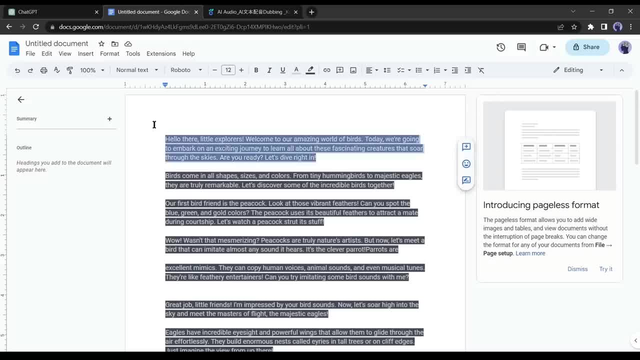 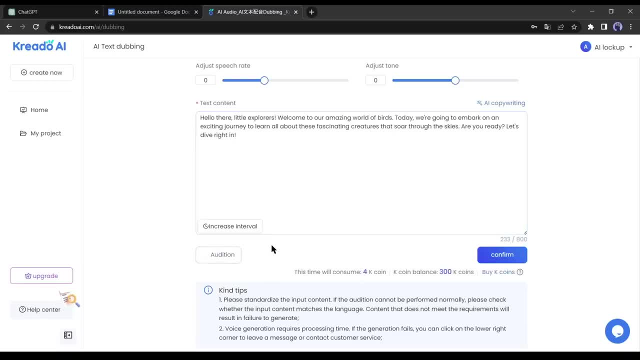 select your preferred language and voice model. Go back to your document file, copy the first paragraph of your script and paste it into the Credo AI text box. Click on Audition to hear the output. Hello there, little explorers, Welcome to our amazing world of birds. If you are satisfied, 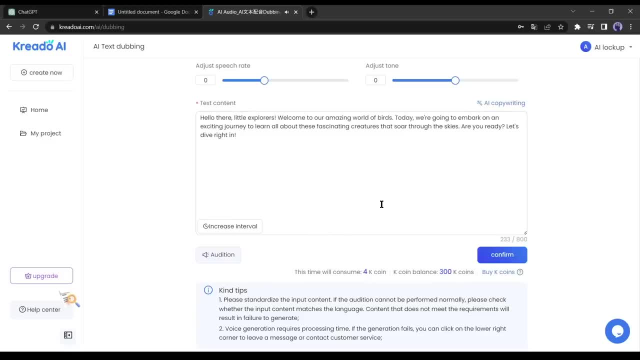 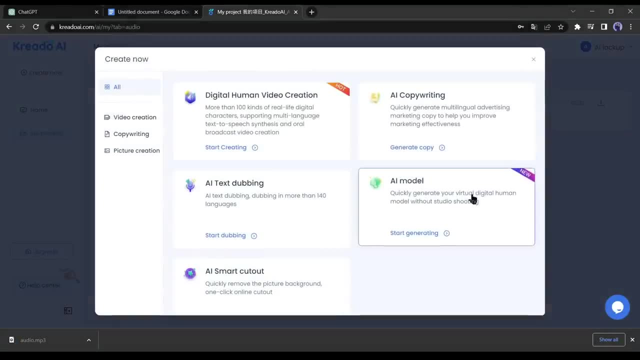 with the voice. click on Confirm. Otherwise, change the voice model and audition again until you are satisfied. Once satisfied, click on Create New and select AI Text Dubbing. Now click on Create New and then select AI Text Dubbing Again. go back to doc file and copy the second paragraph. 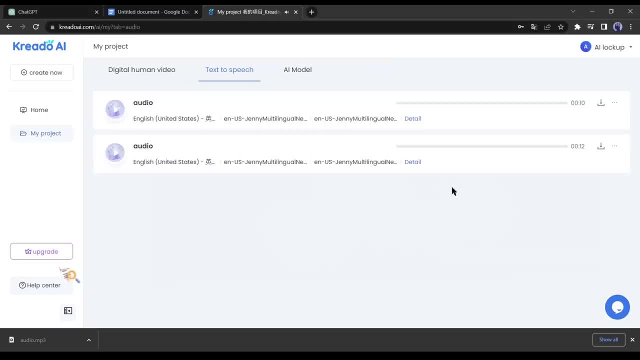 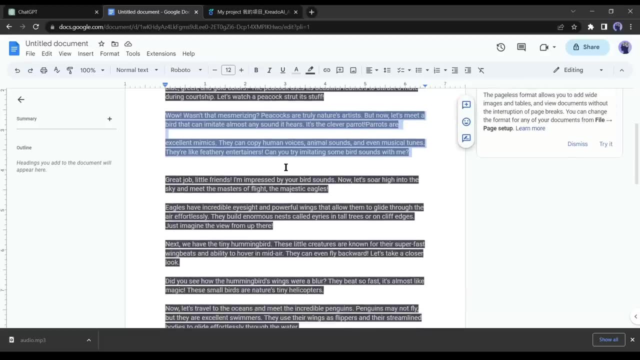 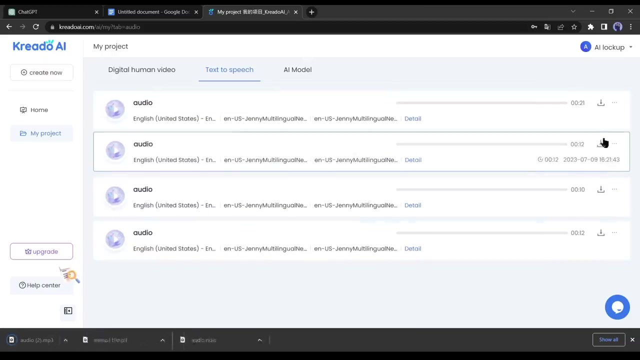 and paste into Credo AI text box. After lessening the output, click on Confirm. Do it again and again until you don't convert all the paragraph of your script. After converting the entire script, download all the audio. This completes our voice generation step. In the next step, we will generate the animated 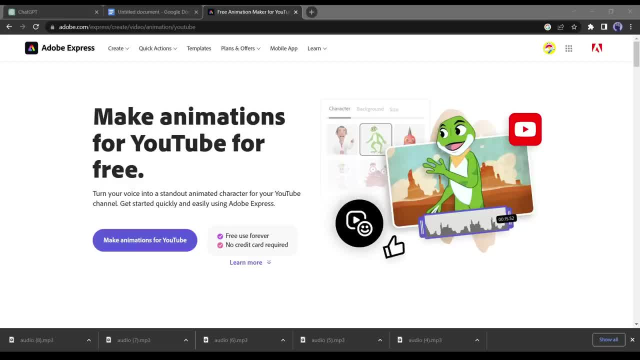 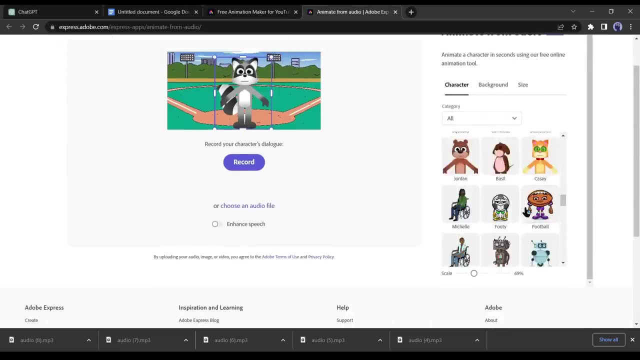 character with the audio. For animation, we will use Adobe Express, a free AI animation tool. Once you are in Adobe Express, click on Make Animation for YouTube. Select a funny character for your video. since we are targeting children and funny characters, keep them engaged. After selecting the character, click on Background. 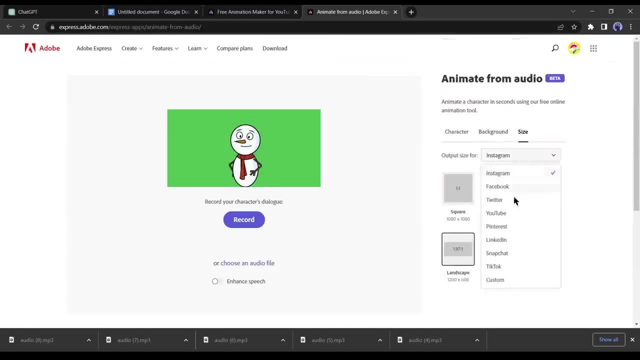 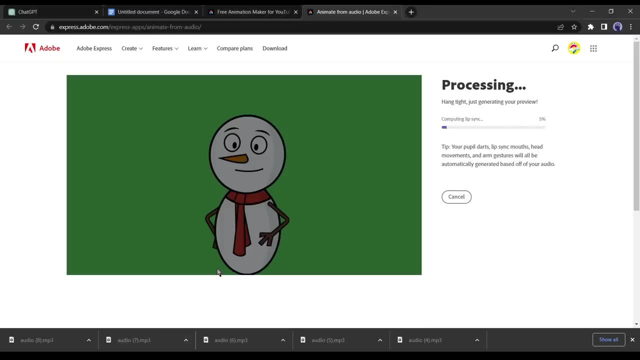 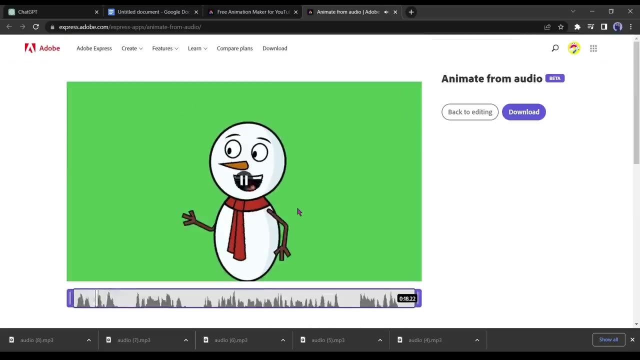 and choose a custom color. Then select the video size as YouTube Video Size. Now upload your first audio clip or simply drag and drop it into the designated area. Adobe Express will take some time to generate the animated character with our audio. Once the generation process is complete, click. 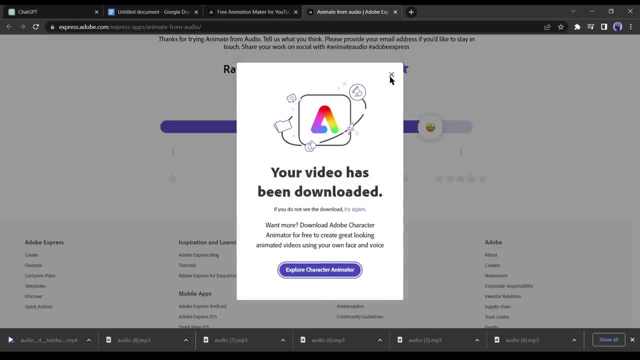 on Download to save the video. After downloading the video, click on Back to Editing, followed by Replace audio. Click on Replace Audio and select your video file. Select the character and select the voice you want to make. Enter the name of the video file you want to make. 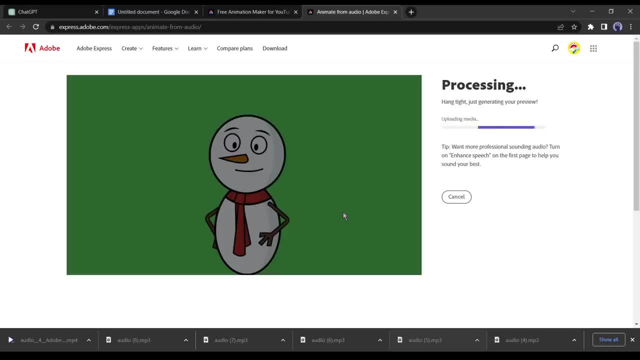 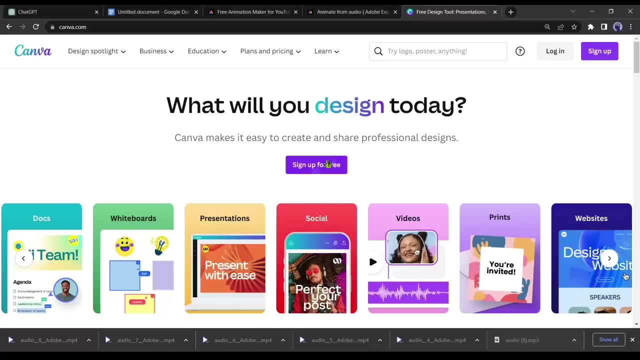 character, change the background if needed and upload the second audio clip. Repeat this process for all the audio clips. This completes our third step. In step number four, we will use Canva to create animated footage for our video. If you are new to Canva, create an account using your email After. 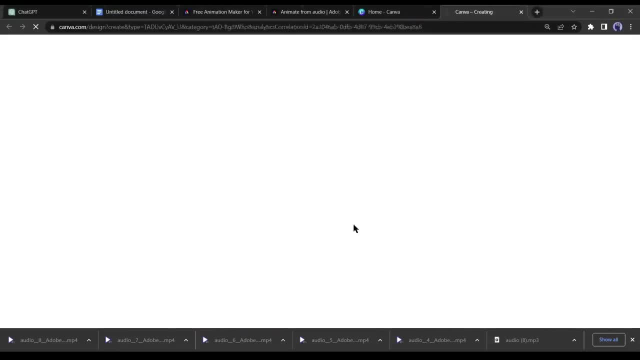 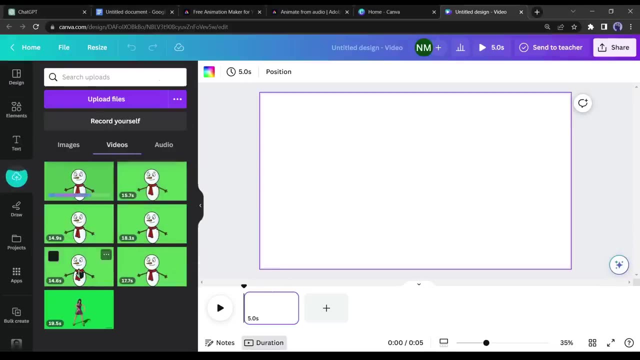 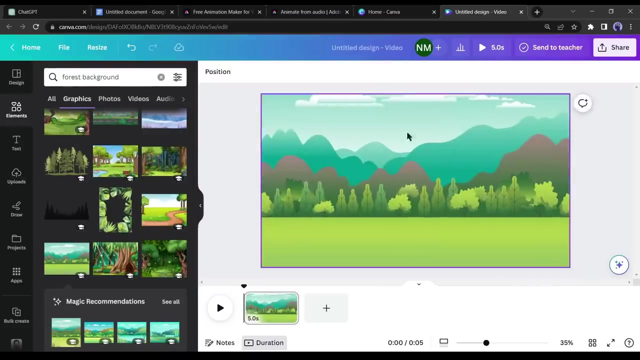 creating an account. click on Video and select YouTube video. Upload all the animated videos generated by Adobe Express. After uploading the animated videos, click on Elements and search for Forest Background. Select a suitable background image and adjust it to the video size. To adjust the video size, refer to the animated video's duration in your Upload folder. 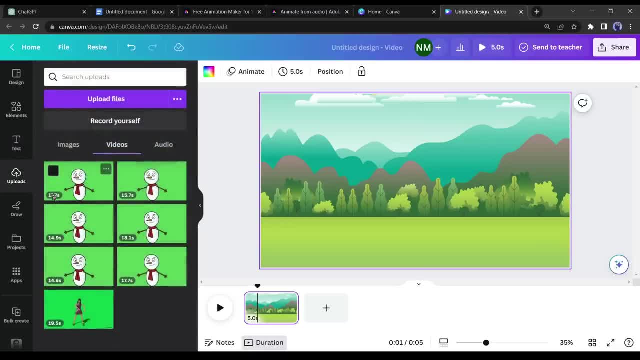 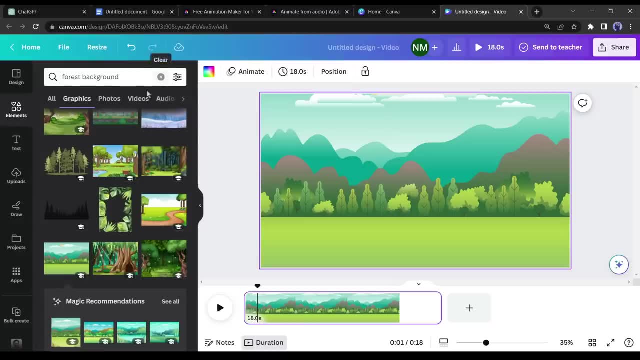 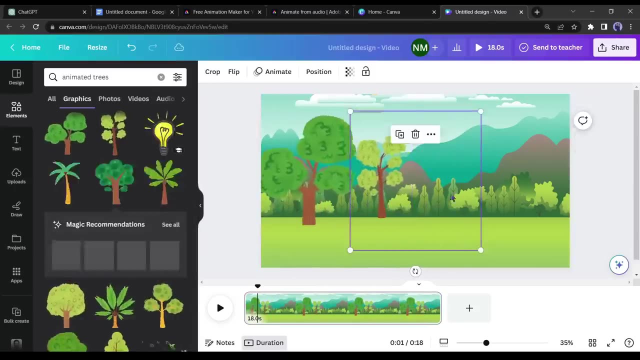 For example, if the first video was around 17.7 seconds, adjust the timer to 18 seconds for perfect synchronization in the Editing section. Now go back to the Elements section and add some animated trees to make the video more visually effective. Search for animated trees, select them and position them in the background image according. 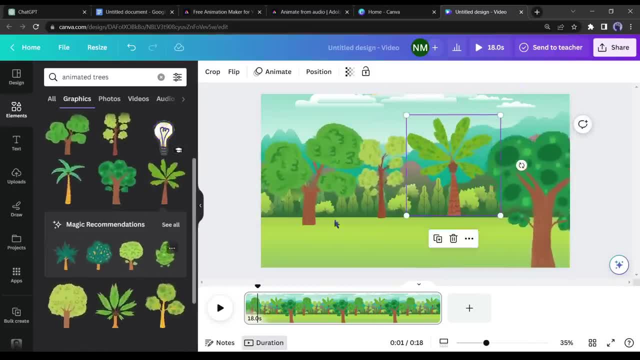 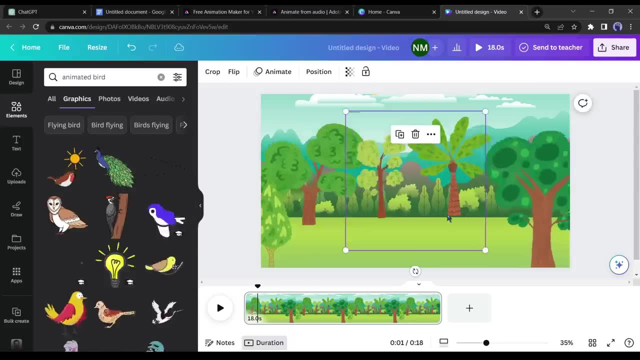 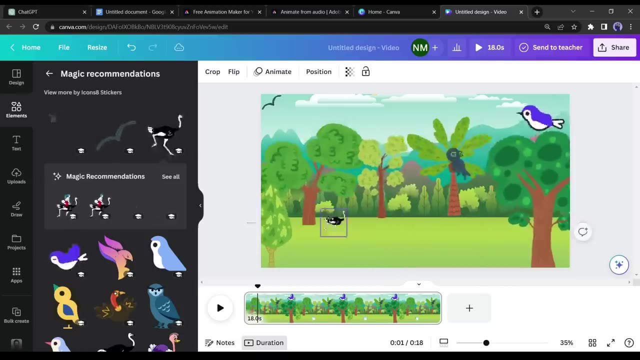 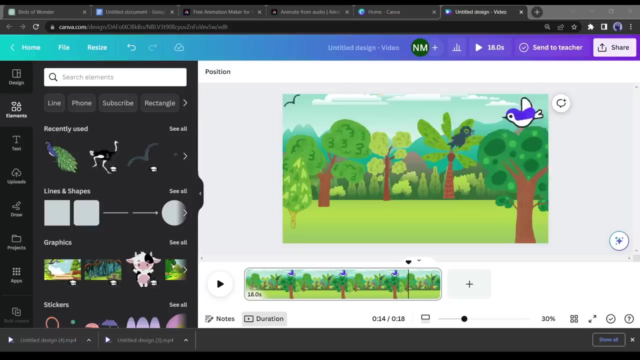 to your preferences. Additionally, add some birds to the video's background. since we are making a video about birds, Once everything looks beautiful, download the background image. Now go back to the Google Docs document and find the first bird mentioned in our script. 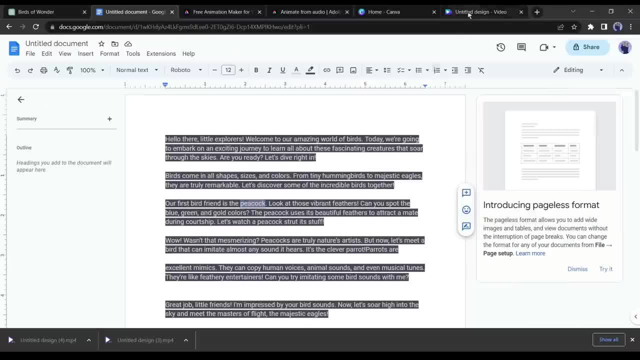 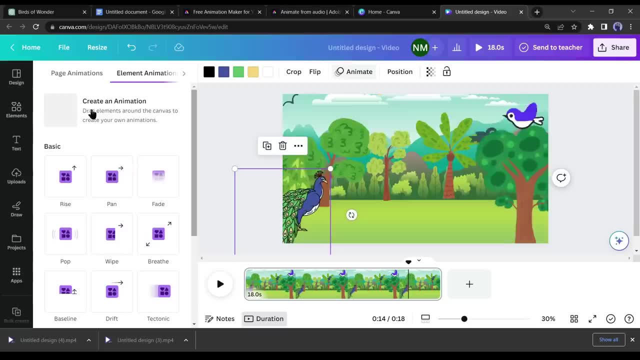 which is a peacock. Return to Canva. search for a peacock in the Elements section, select a suitable image and adjust its size. Here comes the amazing feature of Canva. Click on Animate, then select. Create an Animation. Drag the peacock to the desired position. 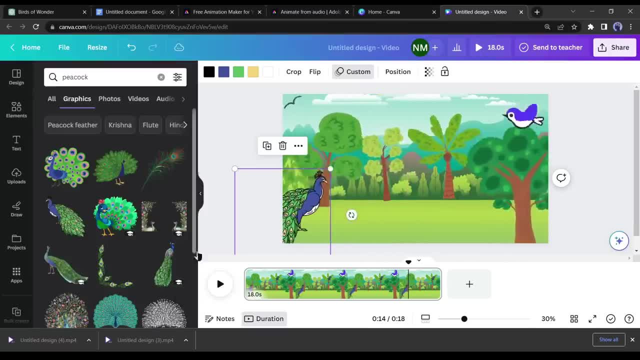 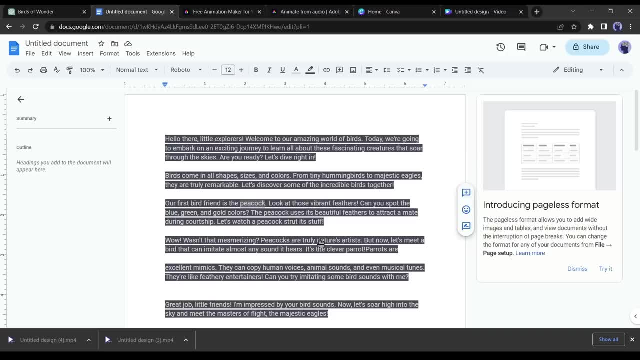 and you will see the peacock moving around in the background. Download the video after making these adjustments. Delete the peacock from the video and add the second bird mentioned in the script, which is a parrot. Repeat this process for all the birds mentioned in the script and. 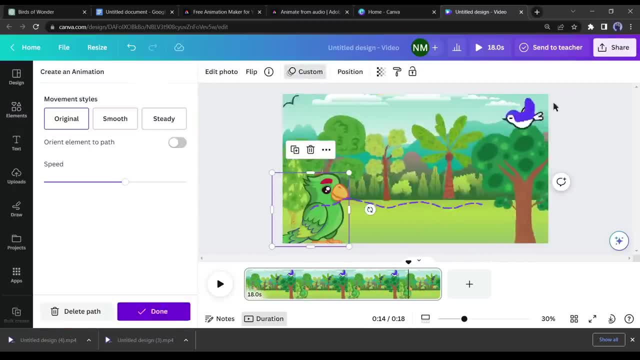 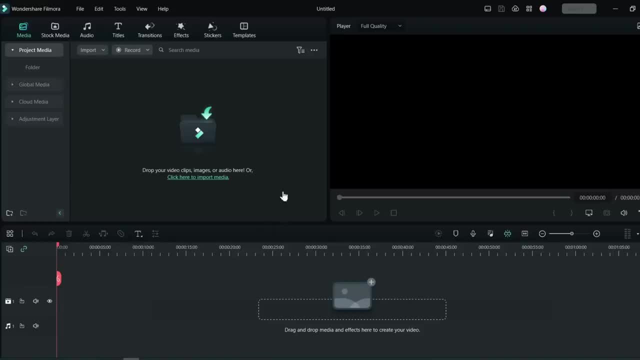 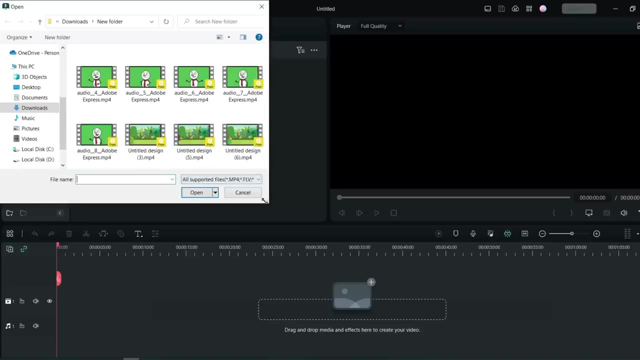 download the videos accordingly. This completes our fourth step. In step number five, we will edit the videos and give the final touch to our video using Wondershare Filmora as our video editing software. You can use any video editing software of your choice, Import all the animated videos and. 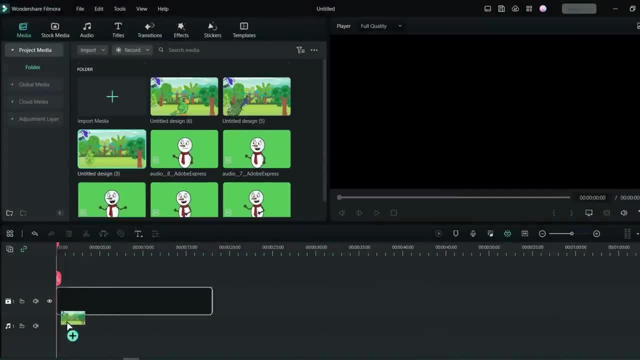 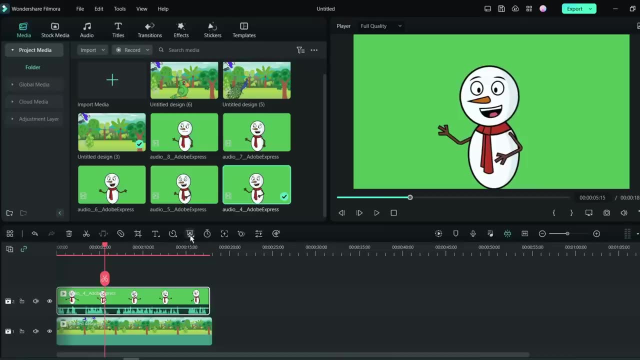 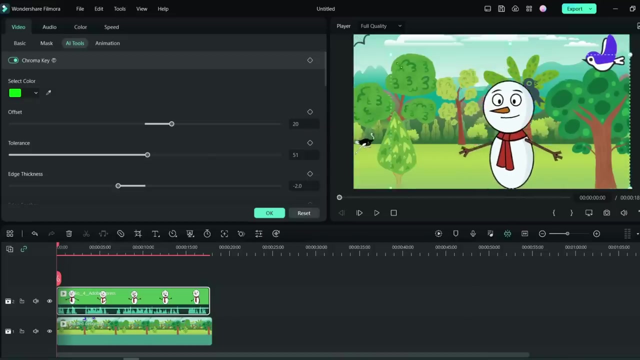 background videos into the software. Insert the 1st background video in the Video-layer 1 and the 1st animated video into Video-layer 2.. Select Video-layer 2 and enable the chroma key function in your editing software. Adjust the animated character's position according to the background. 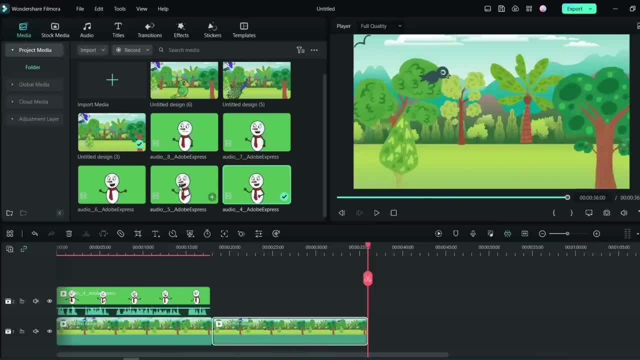 For the second animation, where no bird is mentioned, you can use the same background, Insert the 2nd animated video on layer 2, enable chroma key and allow any bird you want to edit to the 2nd animated video and select the course. 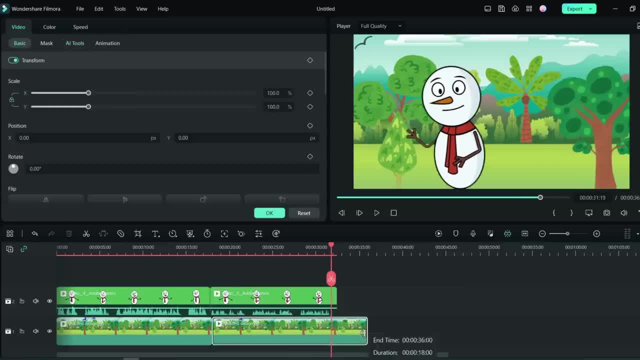 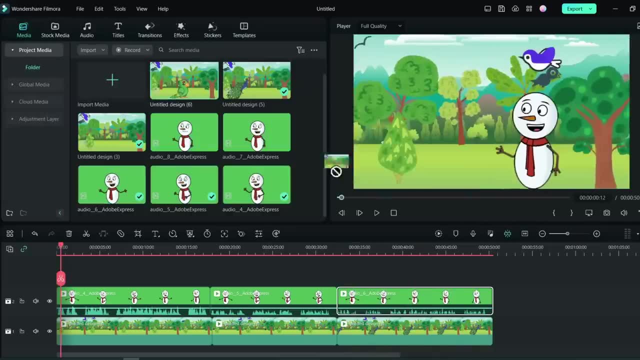 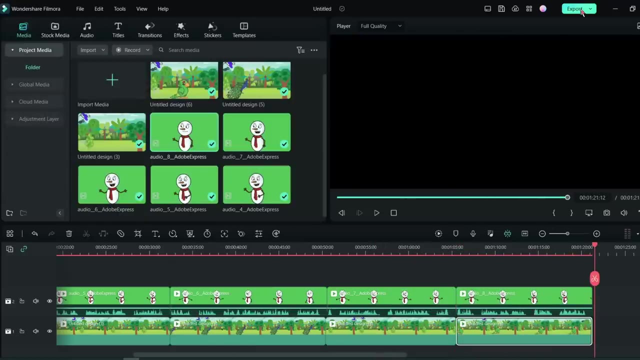 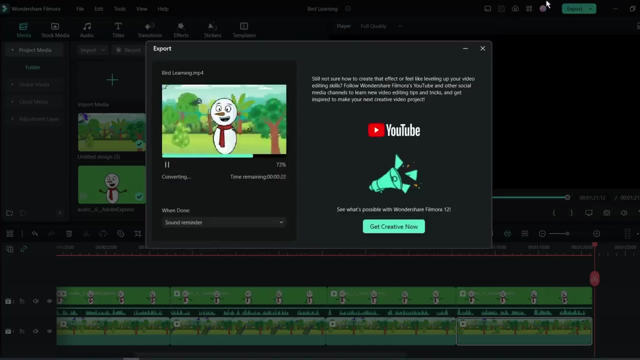 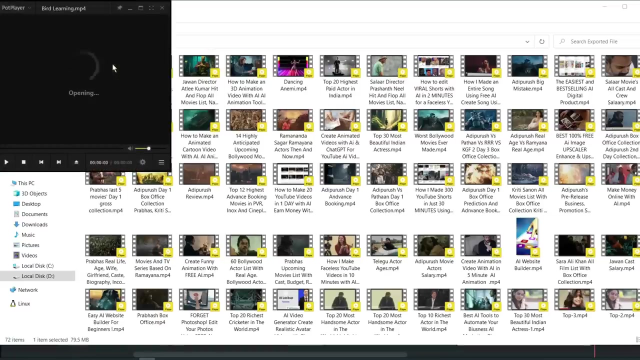 adjust the character's position. adjust the length of the background layer to match the duration of the animated layer. repeat this process for the remaining animated videos. once the editing process is complete, click on the export button to export the final product. congratulations, our animation video is now completed. let's play the video. hello there, little explorers, welcome to our 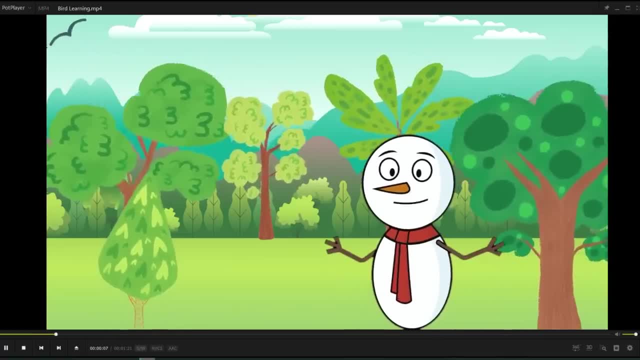 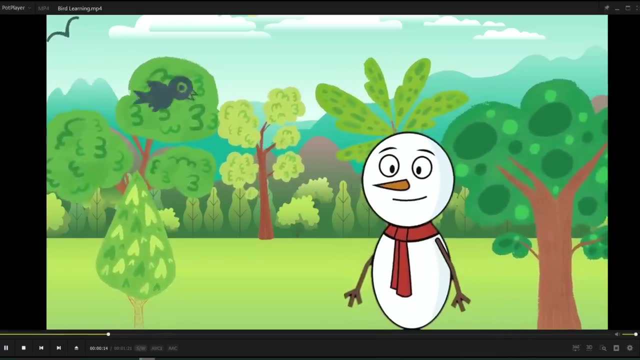 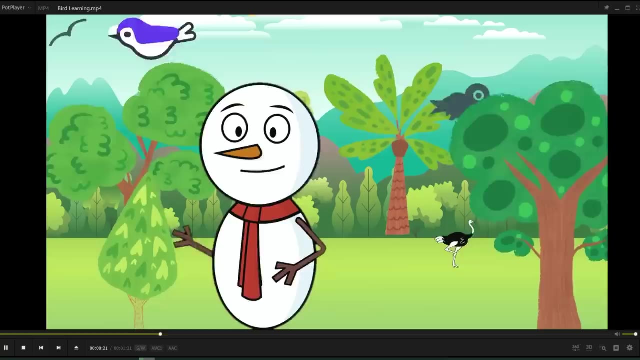 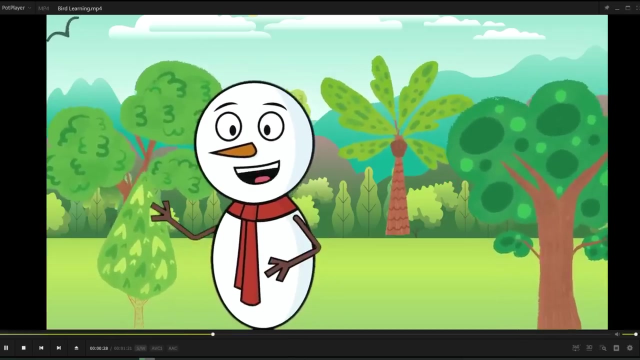 amazing world of birds. today, we're going to embark on an exciting journey to learn all about these fascinating creatures that soar through the skies. are you ready? let us dive right in. birds come in all shapes, sizes and colors, from tiny hummingbirds to majestic eagles. they are truly remarkable. let us discover some of the incredible birds together. 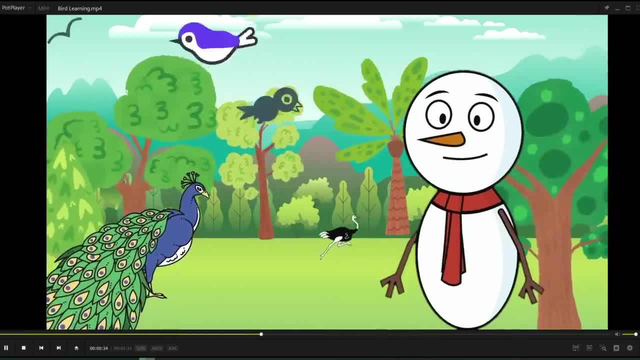 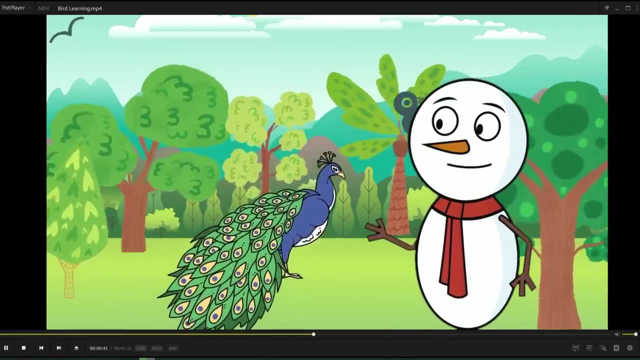 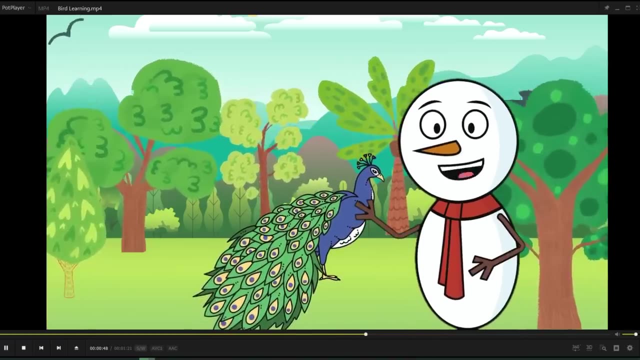 our first bird friend is the peacock. look at those vibrant feathers. can you spot the blue, green and gold colors? the peacock uses its beautiful feathers to attract a mate during courtship. let us watch a peacock strut its stuff. wow, wasn't he that mesmerizing? peacocks are truly.